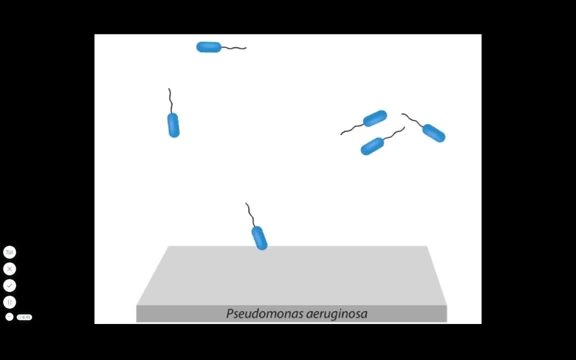 The first stage of biofilm formation occurs when a specific environmental signal induces a genetic program in free-living planktonic cells. In response to the signal, the planktonic cells begin to attach to nearby surfaces by means of flagella, pili, lipopolysaccharides or other cell surface appendages. 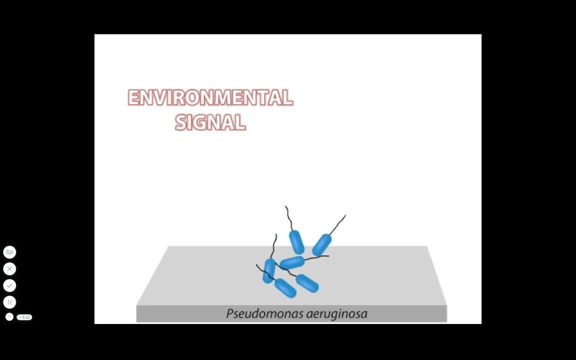 The attached cells begin to coat that surface with an organic monolayer of polysaccharides or glycoproteins, to which more planktonic cells can attach. As the cells enter into biofilm formation, they no longer maintain their flagella. 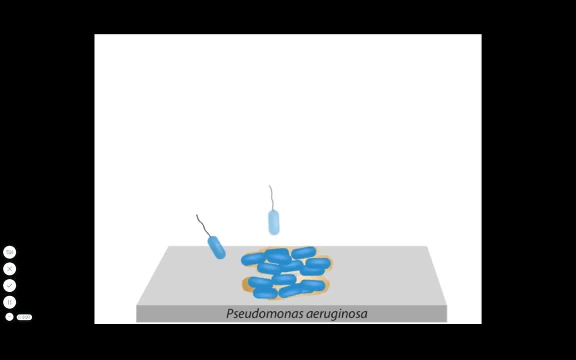 and instead may move along surfaces using a twitching motility that involves the extension and retraction of a specific type of pili. Ultimately, they stop moving and firmly attach to the surface As more and more cells bind to the surface and divide. 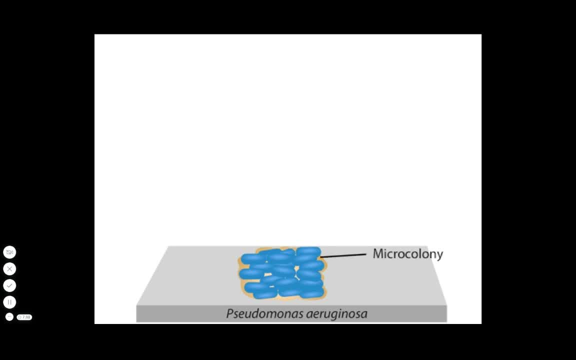 they form microcolonies and can begin to communicate with each other by sending and receiving chemical signals in a process called quorum sensing. These chemical signal molecules are continually made and secreted by individual cells Once the population reaches a certain number analogous to an organizational quorum. 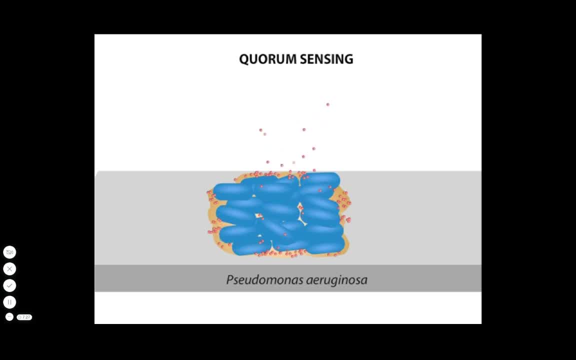 the chemical signal reaches a specific concentration that the cells can sense. This concentration triggers genetically regulated changes that cause cells to bind tenaciously to the substrate and to each other. Quorum sensing may influence the amount of extracellular matrix produced by the cells? 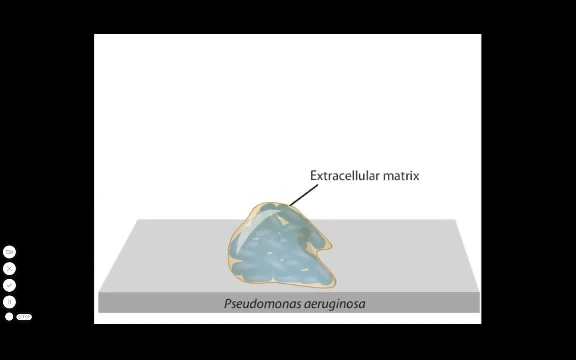 This thick, slimy material consists of polysaccharide polymers called exopolysaccharides, and entrapped organic and inorganic materials. The extracellular matrix protects the cells from damage from environmental assaults. Quorum sensing serves the biofilm in many ways. 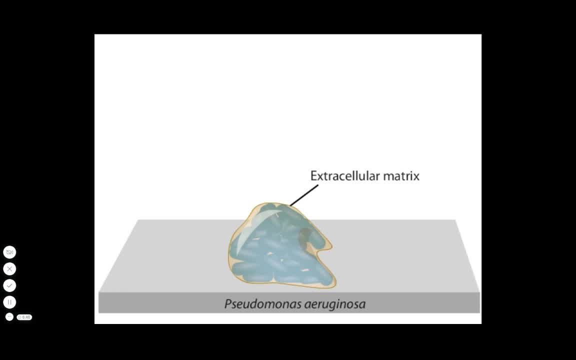 such as by increasing the resistance of biofilms to antibiotics. Quorum sensing in Pseudomonas aerodactyl plays a role in the maturation of the biofilm into complex three-dimensional forms such as columns and streamers, forming channels through which nutrients flow.